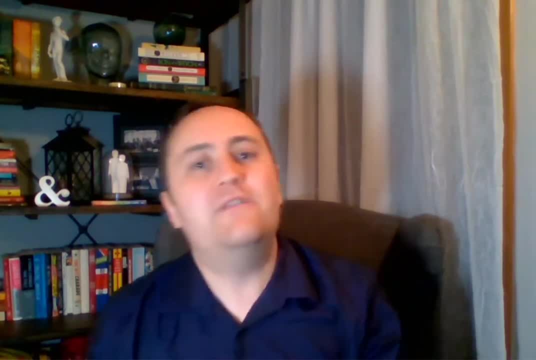 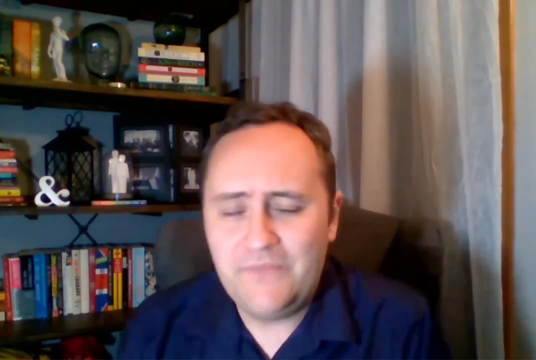 line graphs are a great place to start. They're very, very, very, very common. You've probably seen a million line graphs before. They're very effective, which is one reason why they're common. They just work really well And also there's a lot of flexibility and choices to make You can. 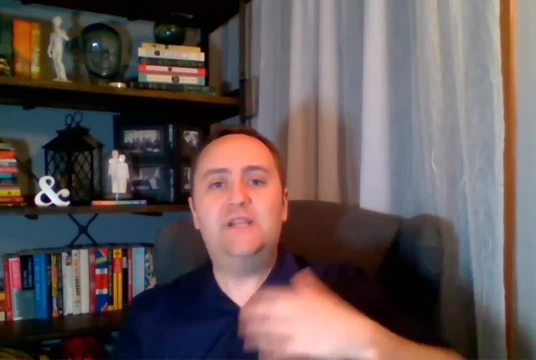 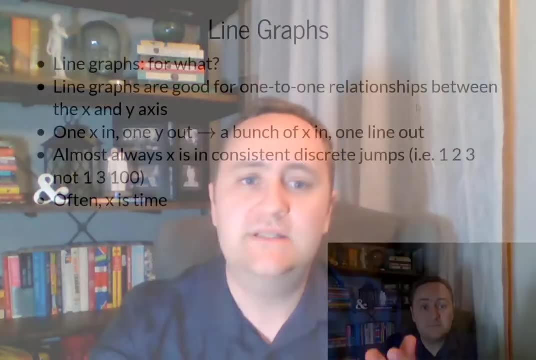 do a line graph very poorly. So let's talk about some of the things that we need to think about when we are making line graphs. So, first of all, what are line graphs good for? What kinds of stories? Well, generally line graphs are good. 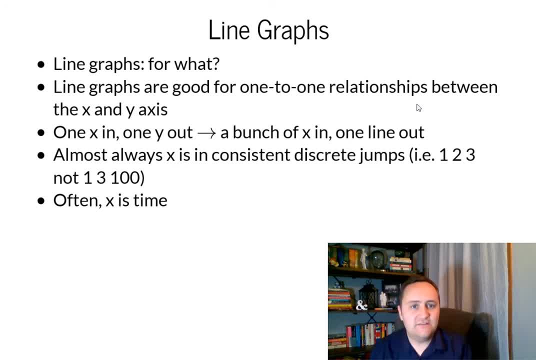 for one kind of thing, Things where you have one x variable in and that gives you one y value out. There's a one-to-one relationship between x values and y values. The x values always go forward. Nothing doubles back, right, You know you don't have an x-axis of 2009, and it goes 2009 to 2010,. 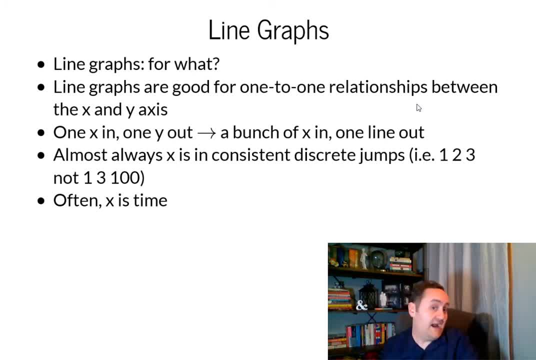 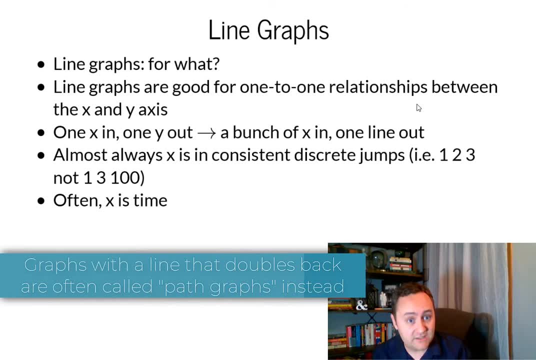 and then back to 2009 again, like that. It wouldn't make any sense for a line graph. It's not what line graphs are all about. Line graphs: you have a single y point for every x point. Now maybe you have multiple lines on the. 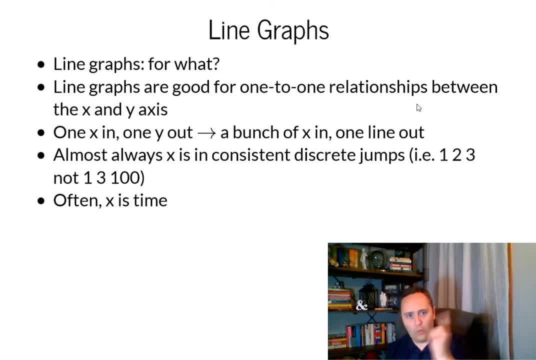 same graph, but every single line has that same relationship: One x in, one y out. In addition, the x-axis should be changing in generally consistent, discrete jumps, So it should be one, two, three on the x-axis, Or January, February, March Or 2019, 2020, 2021.. Things. 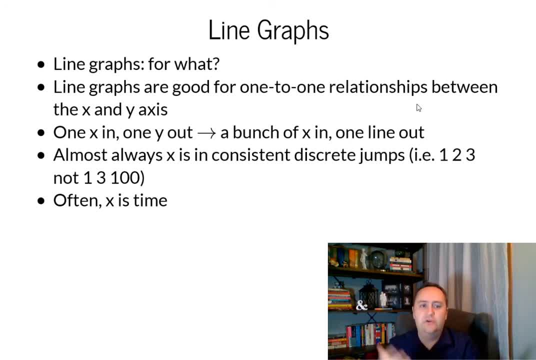 like that. Time is often the x-axis on a line graph, although certainly not Always. It doesn't work quite so well if you have very big discrete or big big jumps in your x-axis between one point and another. It just looks kind of weird to go from one to two to a hundred with 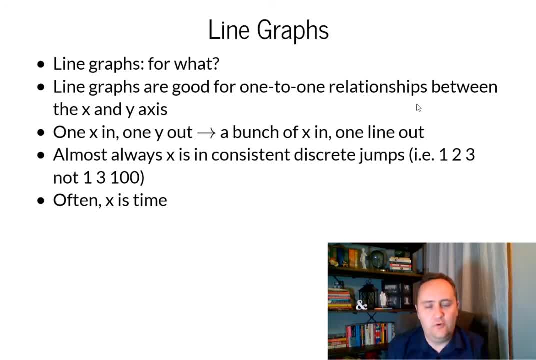 no points in between. So that's the kind of thing we're looking for. Anything where we have a single one-to-one relationship between our x-axis points and our y-axis points, and also our x-axis is discrete and evenly spaced. Those make for the best line graphs. 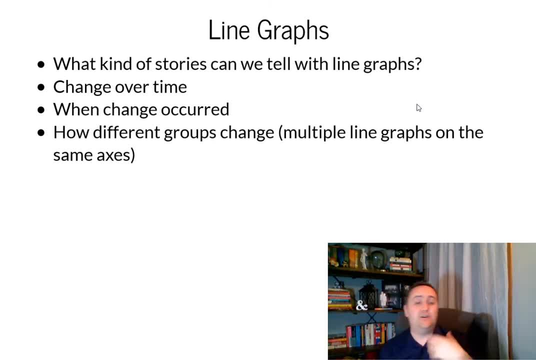 So things that this could is really good at telling Stories, is really good at telling Things about change over time, when that change occurred, And you can also compare different line graphs on the same set of axes very easily, without getting too cluttered to show how different groups are changing over. 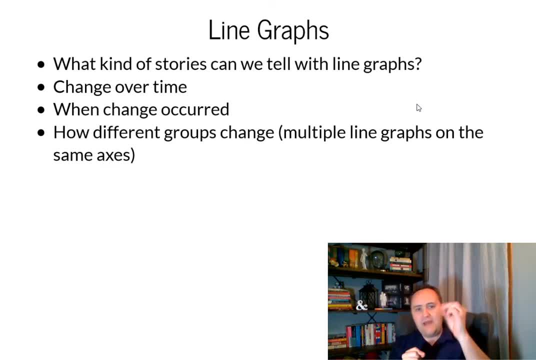 time. So, for example, maybe you have your firm and your competitor's firm and then, over time, you see how your firm is going up and up and up and the other competitor's firm is going down and down and down. That's a very clear story. So, with that in mind, with the kinds of stories that we 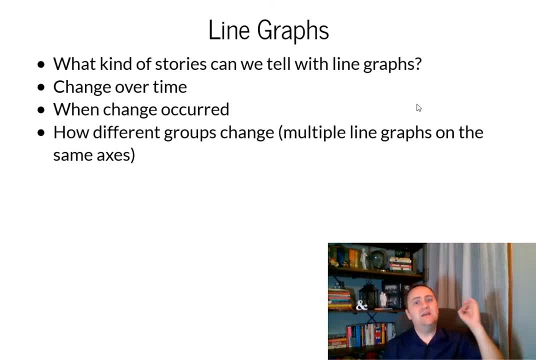 can tell: with line graphs, we're going to go ahead and get started. So I'm going to go ahead and get started with line graphs. How can we do them? well, So the first thing I want to say is: don't be afraid to be really, really simple with a line graph. It's not a waste of space to have a single. 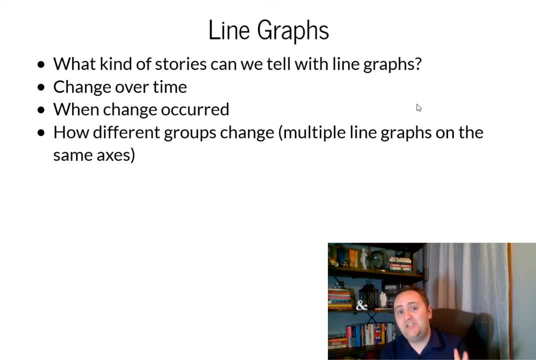 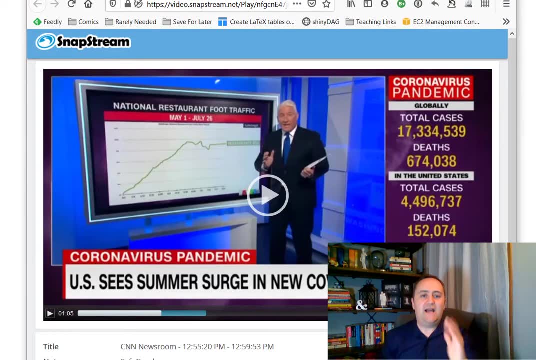 line graph that is just showing you a single number over time, especially if that is telling a very strong story. Let me show you an example of a line graph that I made And, yes, I am showing off. So this is a line graph that I made about national restaurant foot traffic over time from: 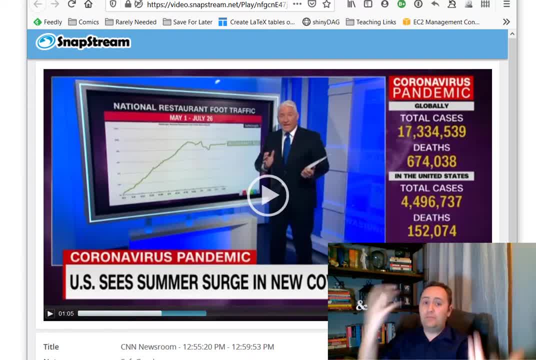 May 1st to July 26th. The question, of course being: are people going back to restaurants During the pandemic? what are we going to see? How would we expect this to affect cases in the future? And so that's the question: Are people going to restaurants? Are they walking into? 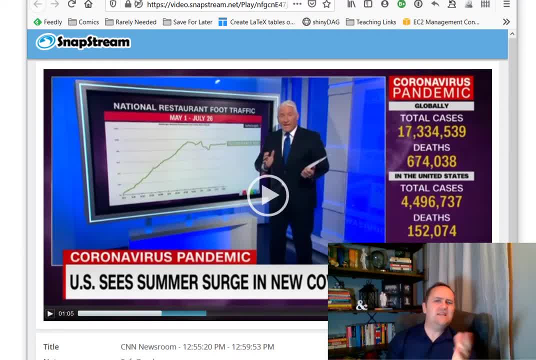 restaurants. Now, this is very zoomed out. You can't see this graph very well from where I'm showing it to you, right? You can barely tell what's going to graph. You can't read most of the text, but still you know the story of what's going on very well. right, As soon as you know. 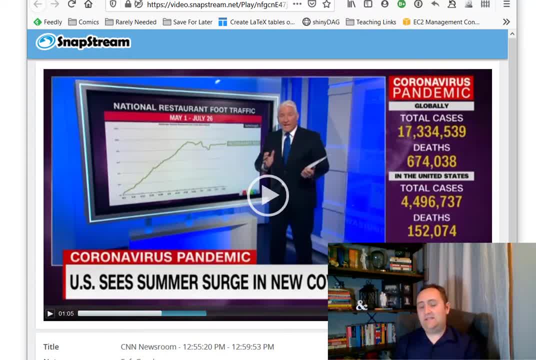 this is restaurant foot traffic. you don't need to read any of the other texts to have a very clear idea of what the story is. There's an upward slope, It gets bigger and bigger and bigger and then it levels out. That's the story: The fact that we can get across so much information without really getting close. 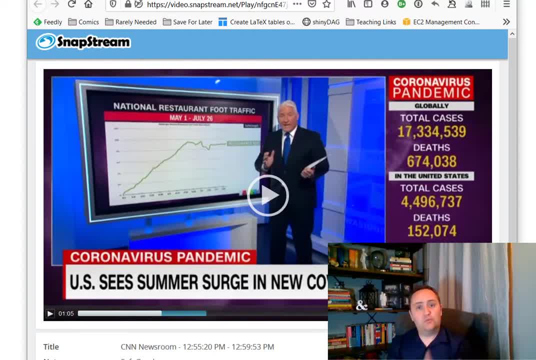 to it, or having good detail in the picture, or being able to read the text from where you're sitting. that's a very powerful graph. So if you have a number that you need to focus on that can tell a story for you, don't be afraid to just put it by itself. You don't need to clutter it up with 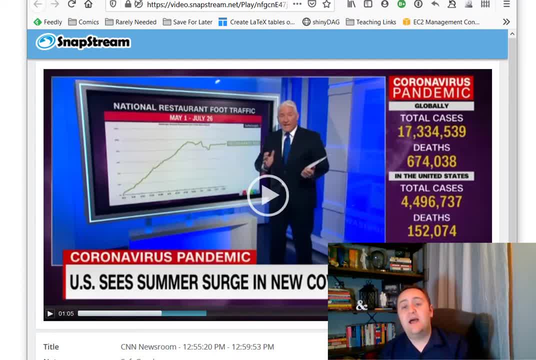 a whole bunch of data points and annotations and everything. A really good line graph can speak for itself. Something else I want to point out here: notice the background here, behind the green line here. So what we have are a bunch of horizontal lines behind the line that we're. 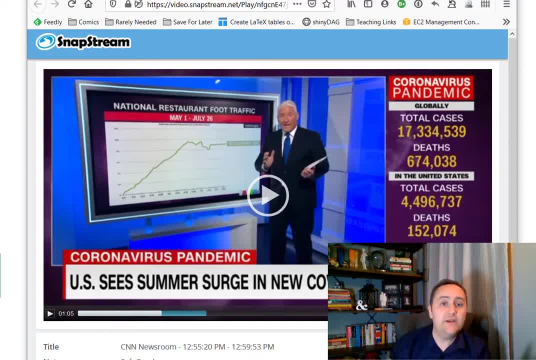 actually tracking here. There's not vertical lines. This is very common in line graphs and in fact a lot of line graph themes that you'll see will use this particular procedure, And the reason for this is on the x-axis we're already sort of marking time or whatever the x-axis is with the 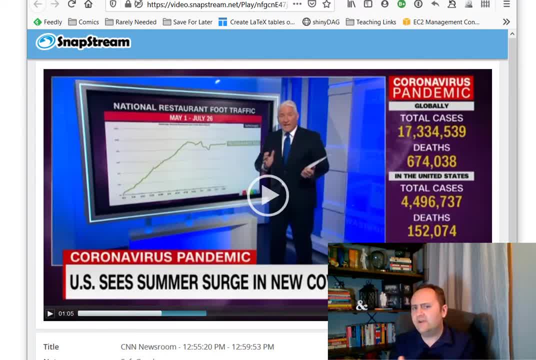 ticks at the bottom And because it's evenly spaced, it's very easy for us to tell sort of where we are in time right, without needing to have a marker in the middle there or even be able to read the x-axis. If you know, this goes from May 1st to July 26th. if you look in the middle of the graph you know. 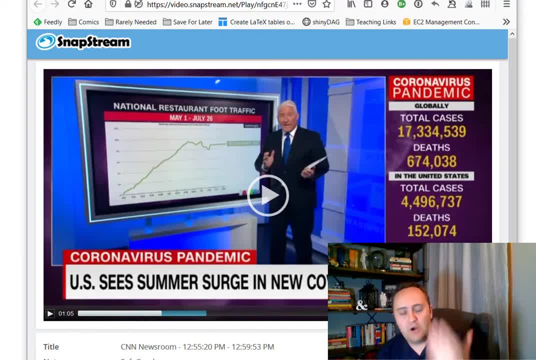 you're somewhere in the middle of June, right, You don't need a marker on the horizontal line to be able to figure that out, But the vertical line is going to be very handy because it makes it a lot easier to tell just sort of how big certain differences are. So, for example, you know. 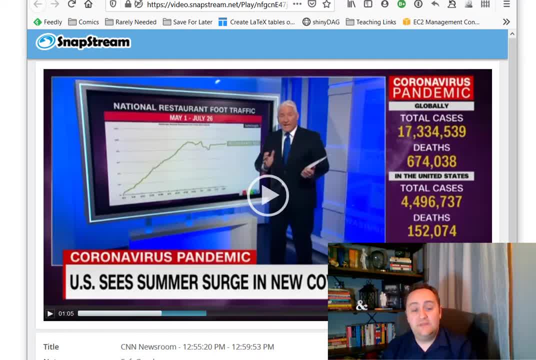 you can see that there's a very straight line On the upswing there with the restaurant foot traffic and that's made a lot easier. It's easier to see that it's a very consistent increase because those horizontal lines are there. The other thing I will point out is that we have labeled the line itself. I'll get a little bit. 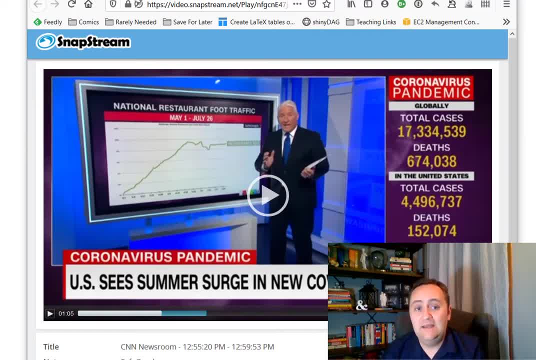 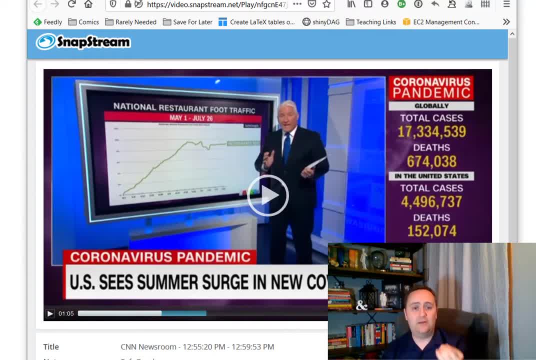 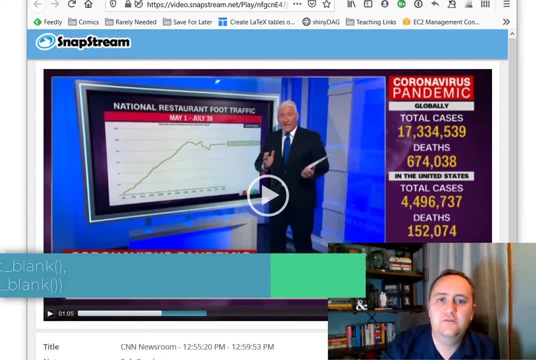 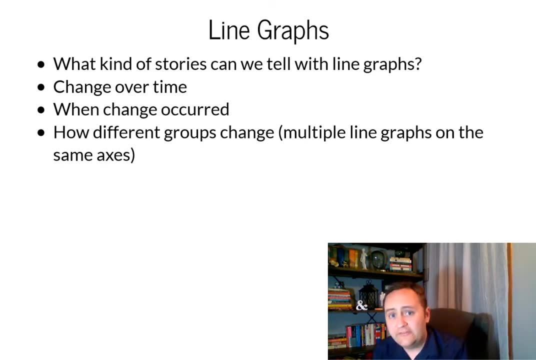 lines you have. with the theme function You can do panel grid axis or panel grid axis. x off equals element blank. That'll work for you. Beyond that, what kinds of things might we think about with line graphs? So often you will have multiple lines on the same graph and also maybe some other. 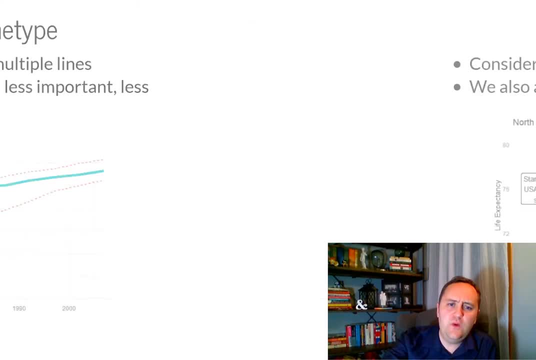 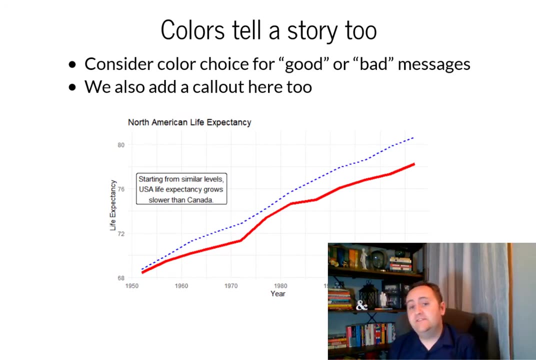 decorations we want to think about. So what do we want to think about there? So if we want to have multiple lines on the same graph, there's a number of different ways that we can distinguish one line from another. Lines lend themselves to a number of different kinds of distinctions. So one is color, an obvious. 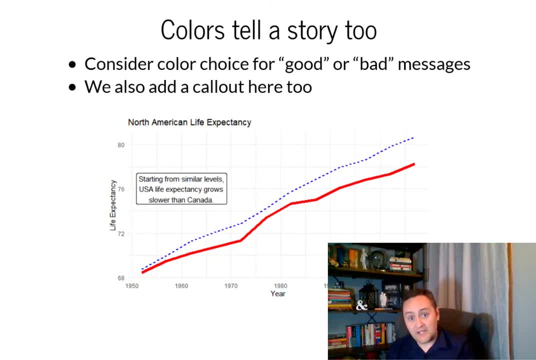 one is color. Again, as always, if you're using color, make sure you're good for colorblind people, that you're using distinct colors that maybe tell a story for you- which ones may be good, which ones might be bad. It can help you out. There's also line type: how many dashes or points? 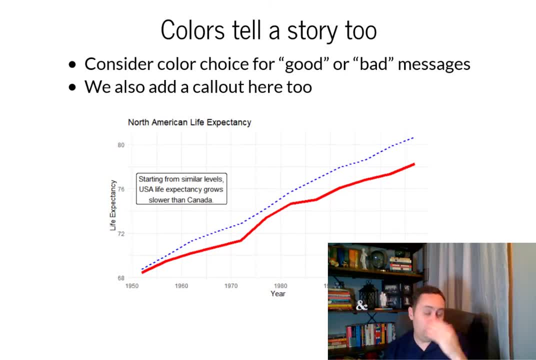 or is it just solid? It can help out. You want to get you know. you can only go so far with that because it's very hard to tell apart one type of dash from another. but you can certainly separate a solid line from a dashed line. That's very easy to do To some extent. you can also do size You. 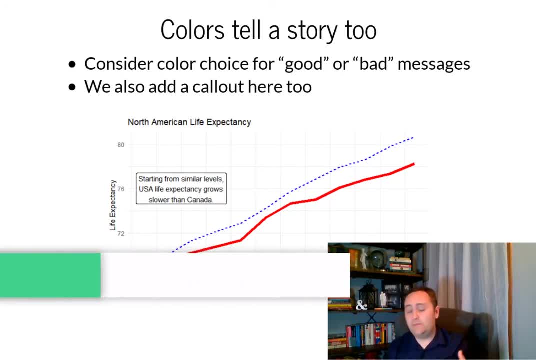 can notice that some lines are very thick, some lines are very thin. If you really want people to distinguish this, you need to go really extreme on the differences. Minor differences in size on lines are kind of hard to see, especially if there's a number of different lines going on. 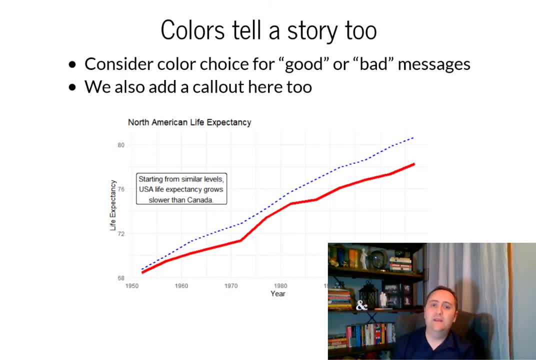 So you can see here one of these lines is at least twice as thick as the other one, and that makes it easy to distinguish those two. So there's different ways we can distinguish different kinds of lines. Another good one is highlighting Often when you're doing multiple 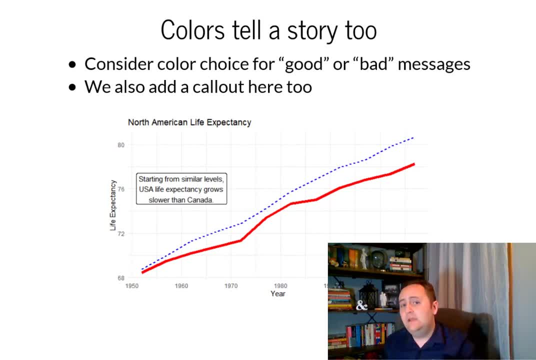 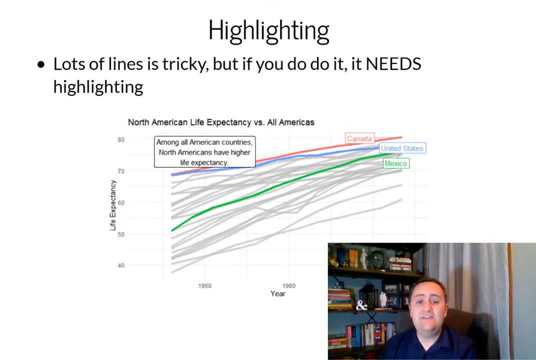 lines on a graph, it's because you're interested in just a couple of them or maybe even just one, but you need some sort of comparison, So for that you can use highlighting. So for example, in this graph here we're tracking life expectancy in North American countries versus 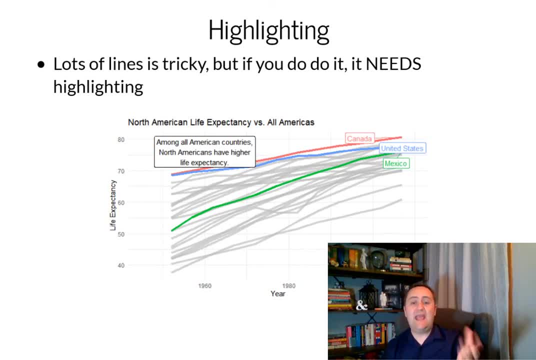 all American countries, And so we highlighted Canada, the United States and Mexico and all the other American countries that are in the background. right, Because all we're trying to do is compare Canada, the United States and Mexico against the rest. We don't need to focus. 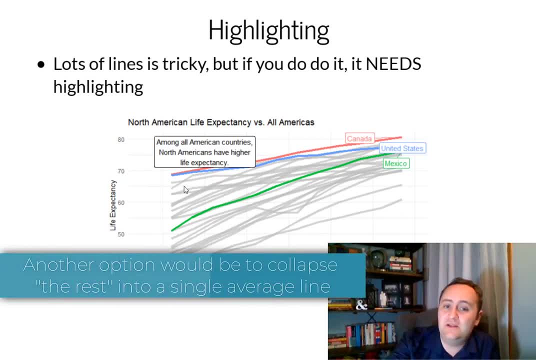 on the rest. We don't even really need to tell apart the rest. Like I can't necessarily be confident in following the rest, I can't necessarily be confident in following the rest. I can't necessarily be confident in following along one of these gray lines from start to end. 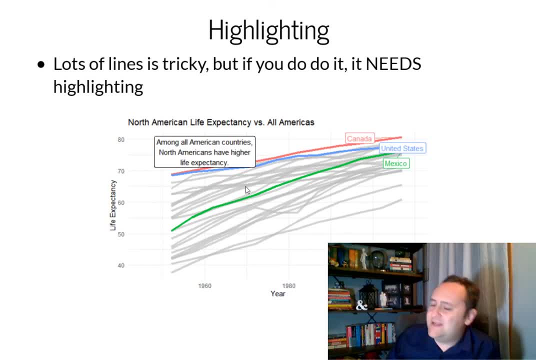 and knowing that I'm following the same one. but it doesn't really matter, right, Because I'm focusing on these ones. in the foreground They're highlighted. Everything else has sort of grayed out and gone to the back. In ggplot you can do this with the gghighlight package. 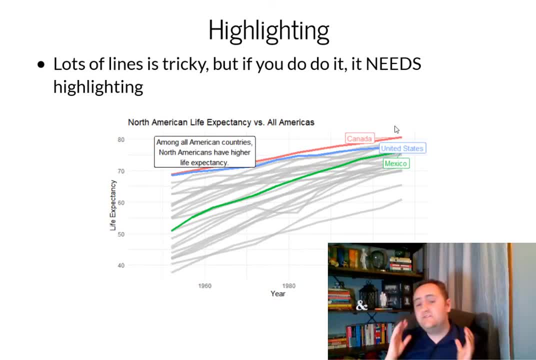 Other good things to note. here I'm labeling the lines. This is very good practice on a line graph. You very, very rarely need a legend on a line graph And in fact, you probably don't want one. Legends are tedious. I don't like them, especially on line graphs, because you have to take the 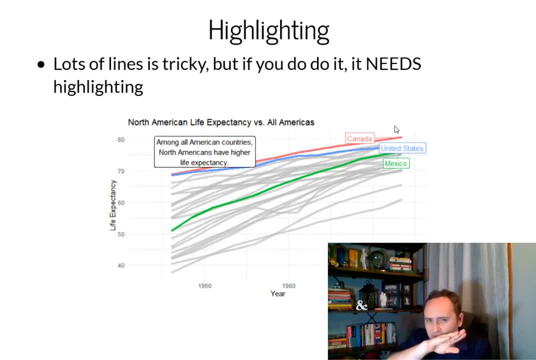 information. that's over there. Okay, the United States is blue. Okay, I follow that over the line. Okay, there's the blue line, That's the United States. It's a lot of work mentally. Or I can just put the word United States on the line itself, Even if you're doing just a single line. 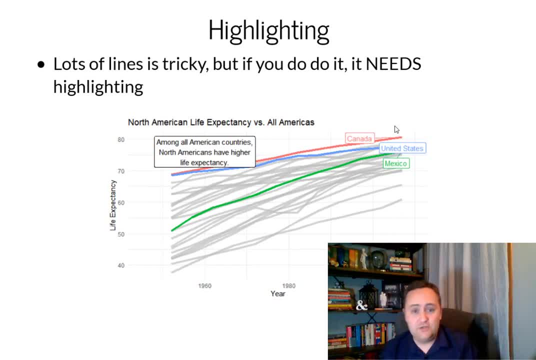 and you don't necessarily need to label things. you could just put it in the title. It's still a good idea to put the label right on there, like we have the restaurants on the on the on the CNN graph, So that's a good idea as well. You can do that in in ggplot using either the. 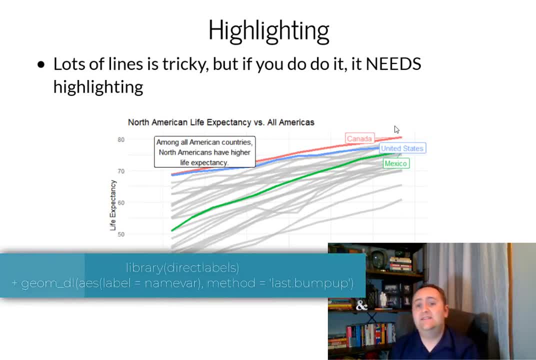 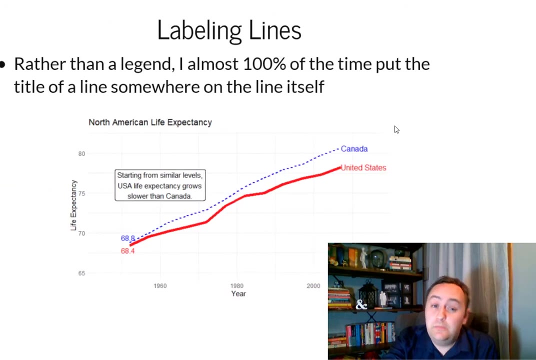 direct labels package or you can use a geomtext to or geomlabel or ggrepel package to to label the last point or the first point of the line itself. That's a good thing as well. Other things to think about here is labeling points. You can label points in line graphs. That's very common. 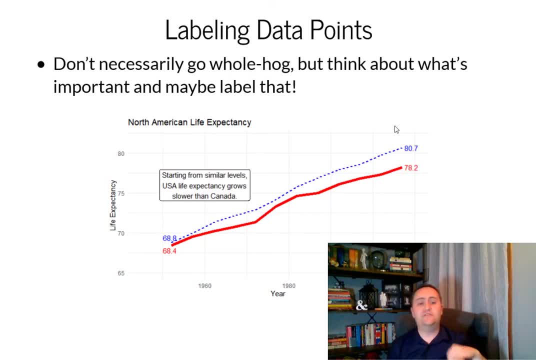 So, for example, here I've labeled the first and last points. on the graphs You can sort of see the values that it's going from. And two: this is nice because it means you don't need to go back to uh the, uh the axes to try. 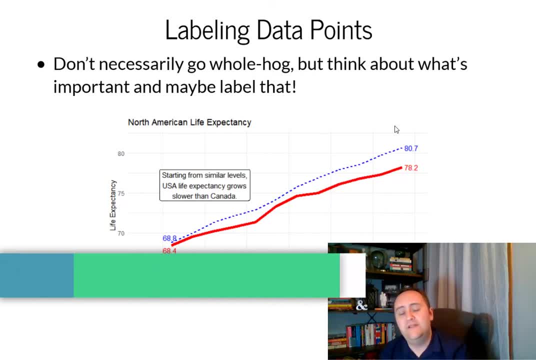 to follow a line along right. You don't need to do that. You're going to see what the point is right there. You can, of course, label points in the middle as well. Again, this is with geomtext and just labeling the first and last points. Uh, it's a. it's a good idea, especially if you need. 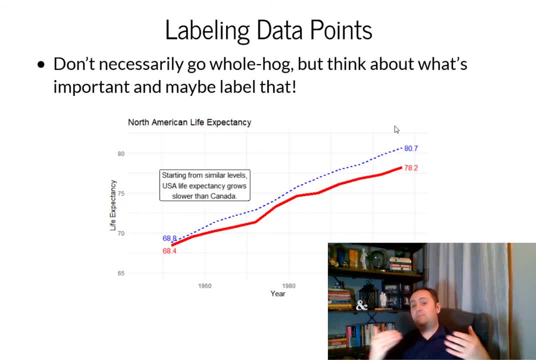 if you need people to know those points, you should put the numbers on there right. Take the information that people need to know. put it on the graph. Don't make them work hard for it. Don't make them follow along to the line to the left. If they don't need to know it, don't put 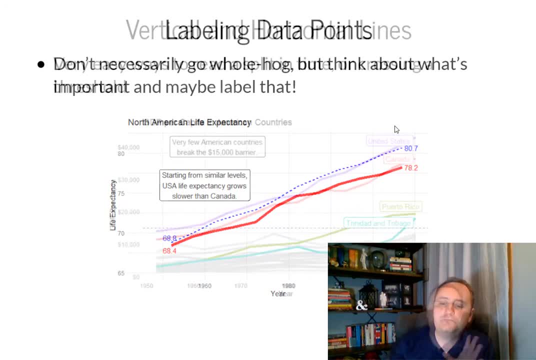 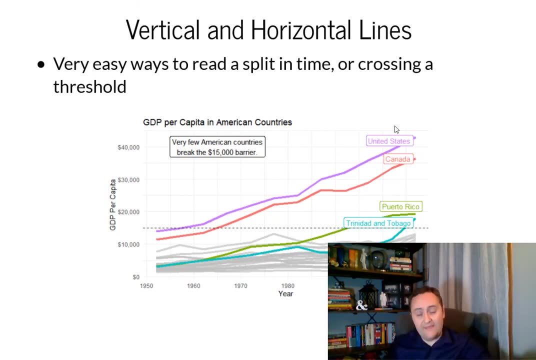 it on there, right? No point Labeling something that you don't want people to know. The other thing I'll point out is that adding horizontal or vertical markers, uh, can be very handy, especially if there's a particular uh border line that you're interested in. So, for example, in this graph I've had a horizontal line. 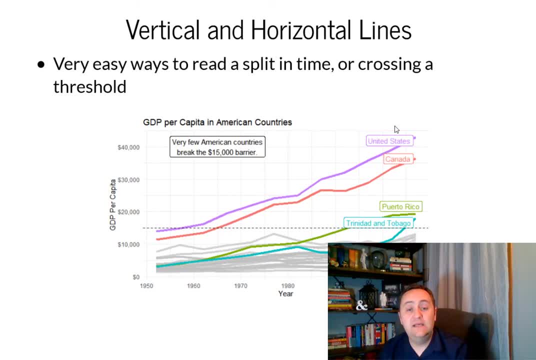 so you can see when lines cross that horizontal line. Uh, so I want to say hey, when do we rise above this particular threshold? Well, it's when we pass across this horizontal line. I can distinguish it from the other lines on the graph by making it dashed and making everything else. 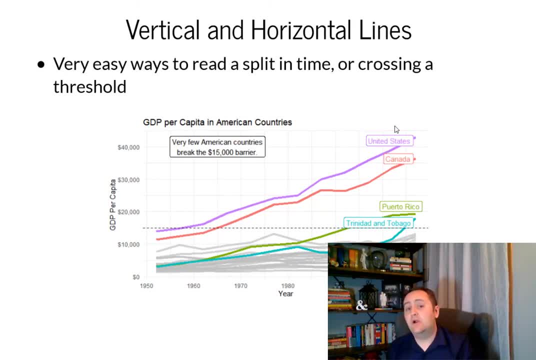 solid, So you can see that I'm not plotting data there. That's a demarker that I've put on by myself. Uh, in this case it also goes beyond the end of either the any other lines, So that also sets it apart, So you can tell that it's not data there.